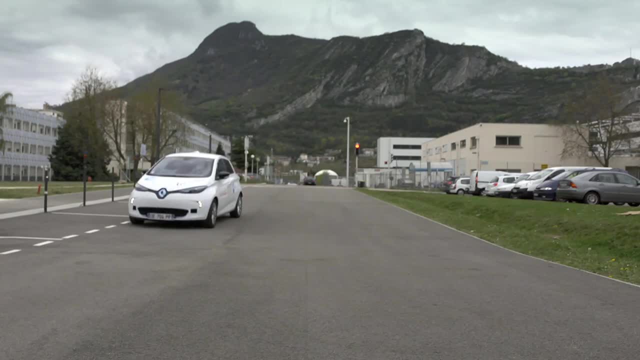 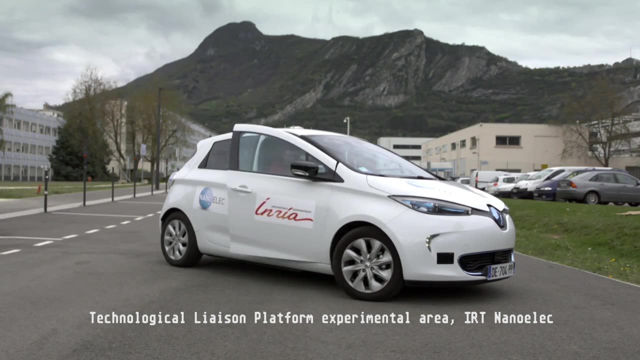 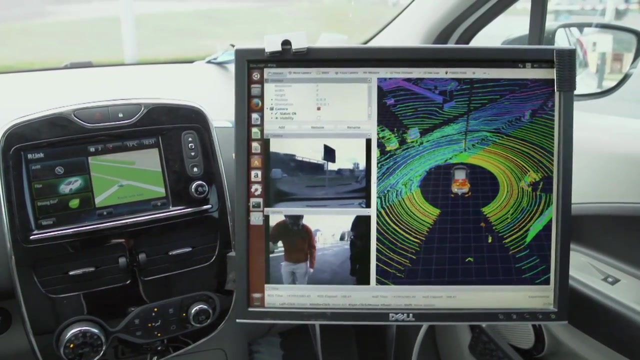 Then the other approach is to conduct actual scale experiments, both on the IRT NanoELEC platform, with our experimental vehicle, but also with some measures taken in the city in order to have access to much more complex environments, In fact, in order to innovate in the area of communicative vehicles. 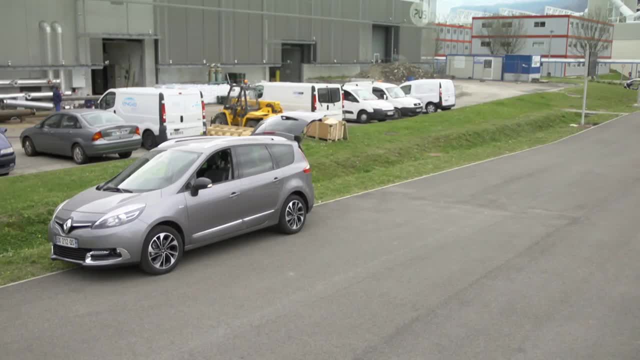 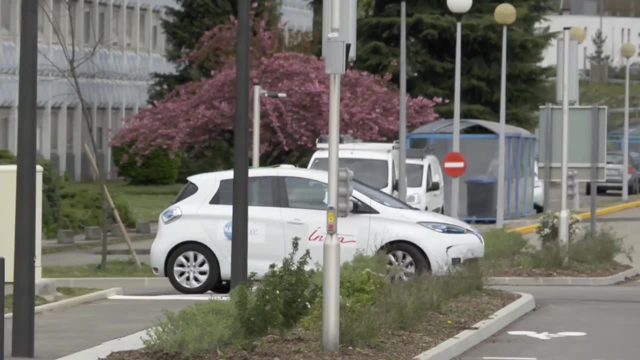 you have to have a test vehicle, a vehicle which is a test platform, but you also need a particular infrastructure so that the vehicle can communicate with the different elements which are those of its usual surroundings, such as interactive street furniture, signage, the road, car parks and barriers. 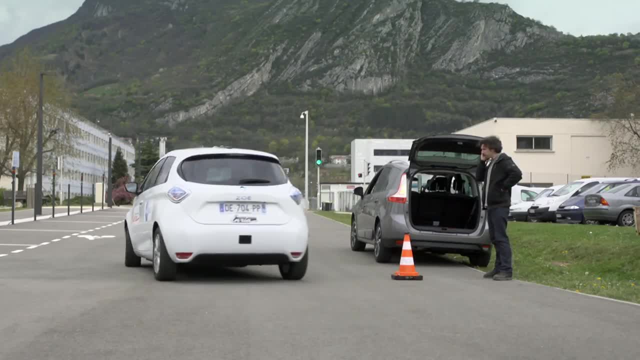 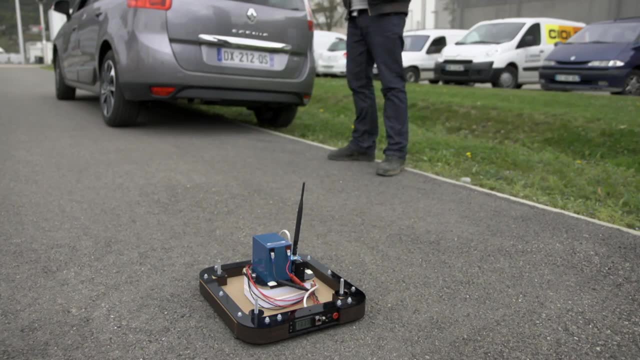 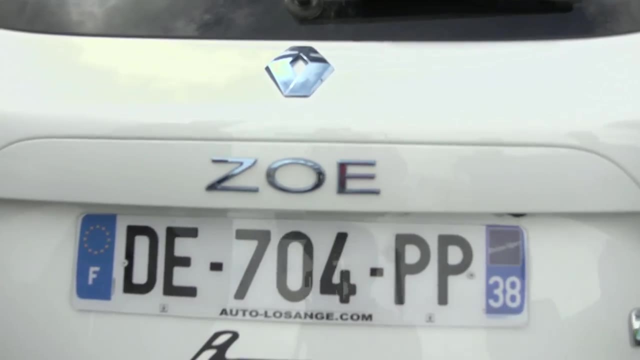 And as it's difficult to gain access to test zones for security or regulatory reasons, in order to validate the performance of experiments that you're carrying out, it is necessary to have a location where you can perform these tests, as is the case with this technological liaison platform. 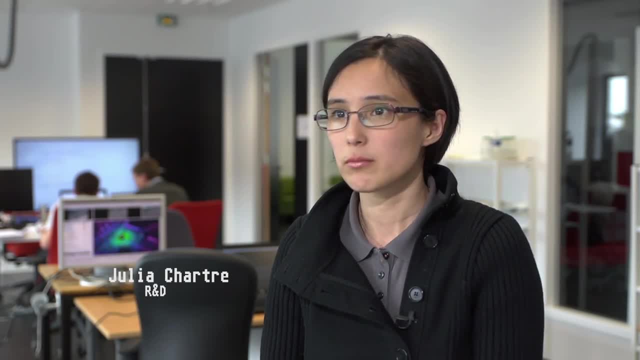 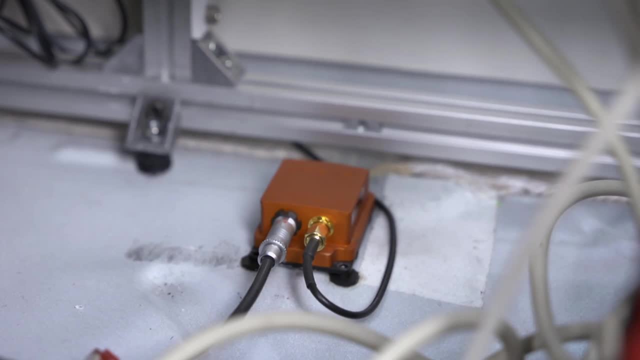 We have a Renault Zoe which has been fitted with sensors. We have rather generic sensors in the car at the moment, such as GPS and inertial navigation systems, which tell you where the vehicle is and what direction it's heading in, But the specific nature of our work is that we use LIDARs. 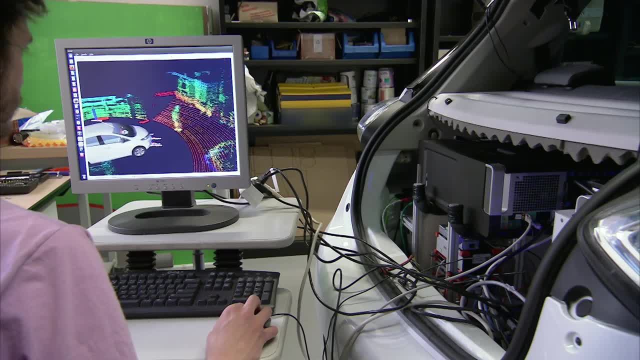 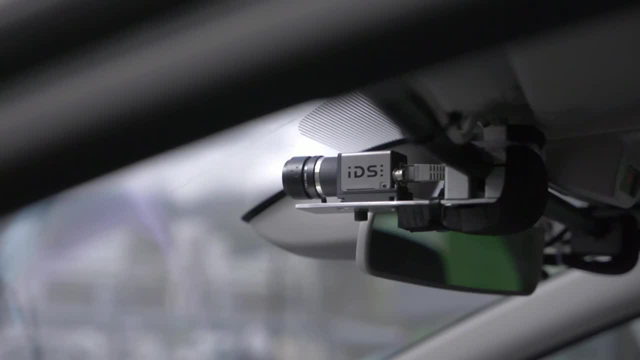 rather like radars, but using light, That's to say that reflections from the light, the same lasers, tell us where objects are in relation to the vehicle. So we also have cameras, one which points forward and one which points backwards, Once our LIDARs have detected an object in space. 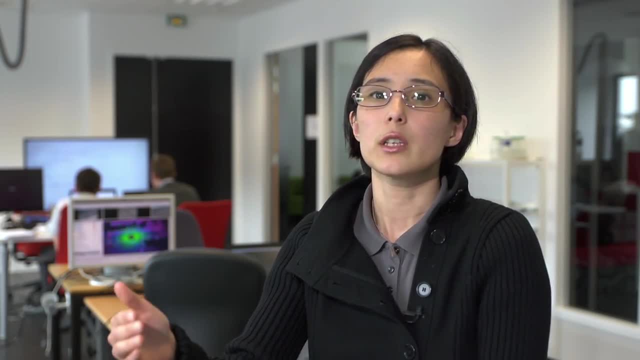 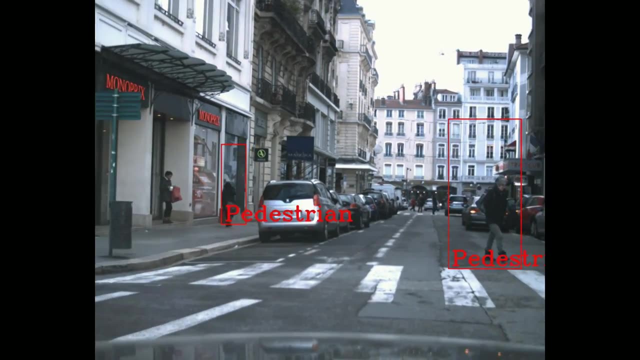 our cameras will help us to identify what it is- whether it's a pedestrian or a bike- And for that we use artificial intelligence technologies on these video images. All these sensors produce mixed data which arrive at different points in time. The idea is therefore to synchronise and merge them. 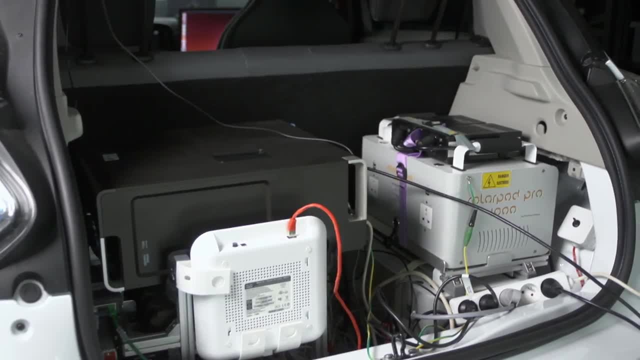 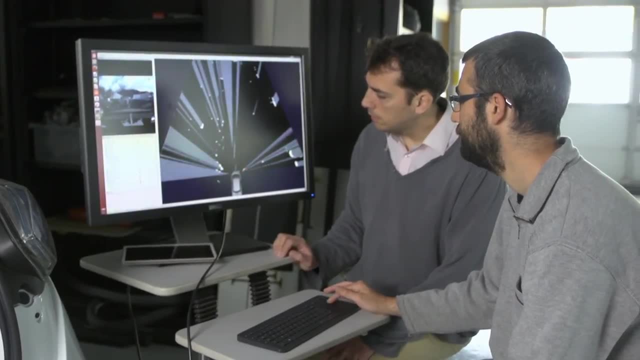 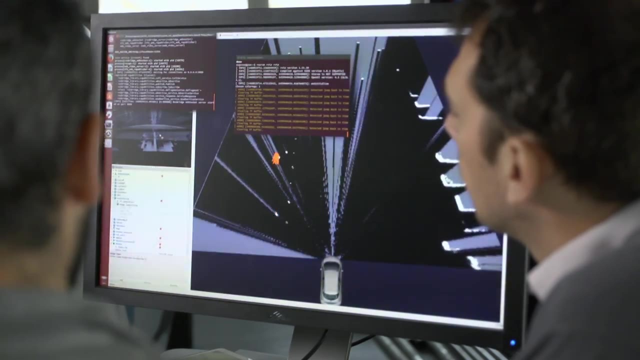 in order to achieve the same results, We need to be able to understand the urban space with these e-mobile and mobile obstacles, and to do this over time. So the first phase for that is knowing how to represent this space, which will be represented by probability grids. 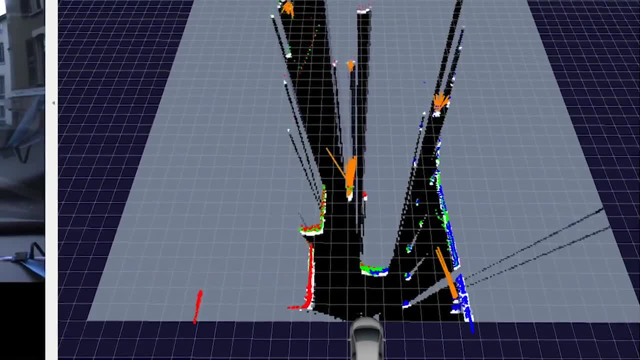 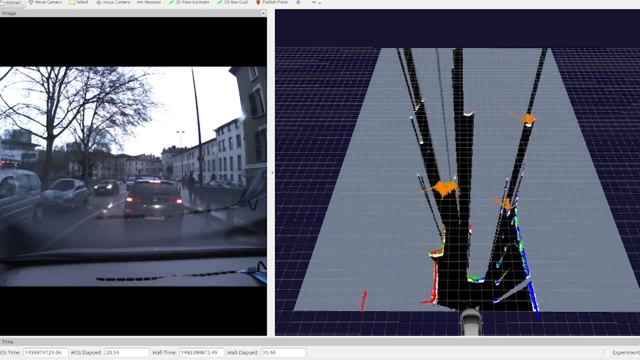 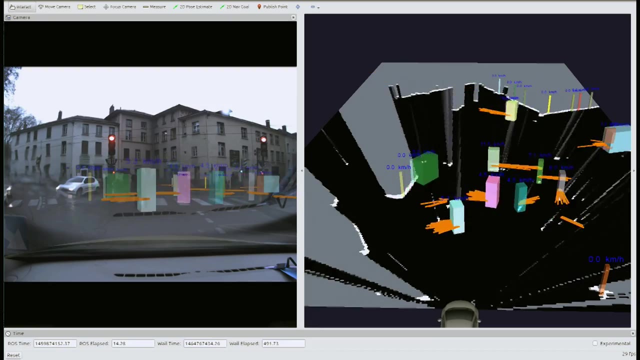 A bit like an image, is represented by groups of pixels. Here we have elements which represent probability of occupation, that's to say the static part of the environment which is detected that doesn't move, And then also probabilities of speed, which measure how things move within this space. 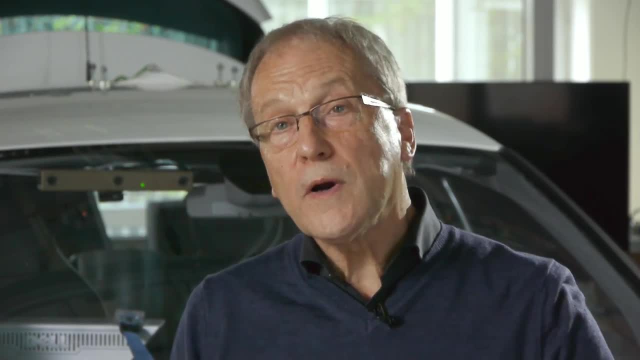 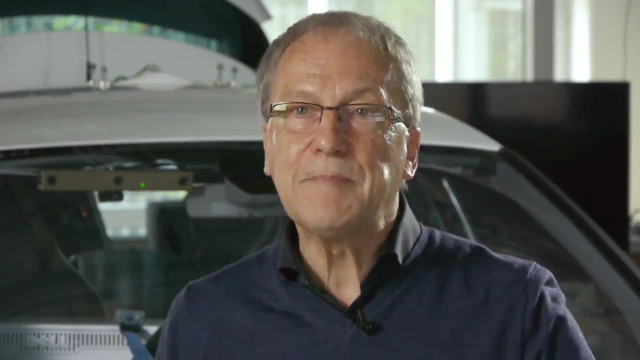 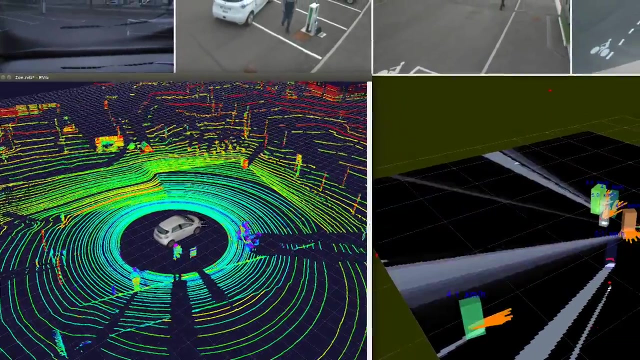 The second principle which we implement is being able to reason about this dynamic space. For that we have developed spatio-temporal reasoning models. This allows us, on the one hand, to extract everything which moves, to extract information on their speed and any changes over time. 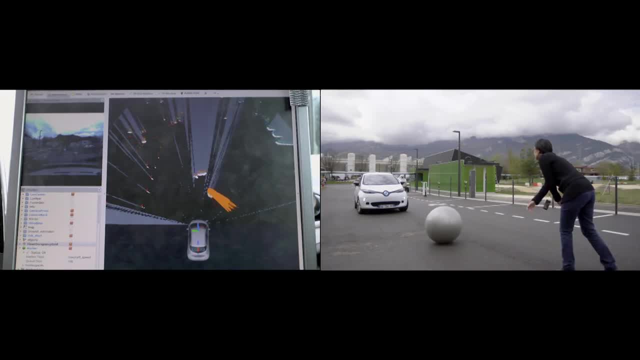 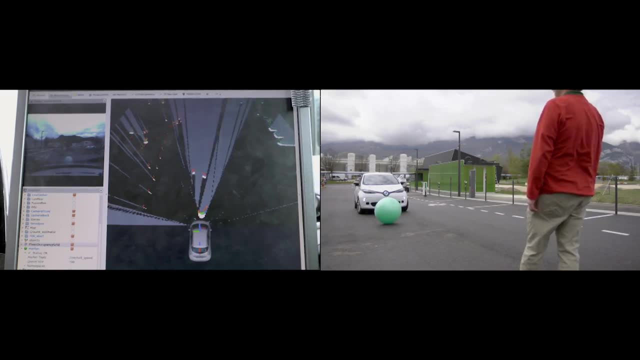 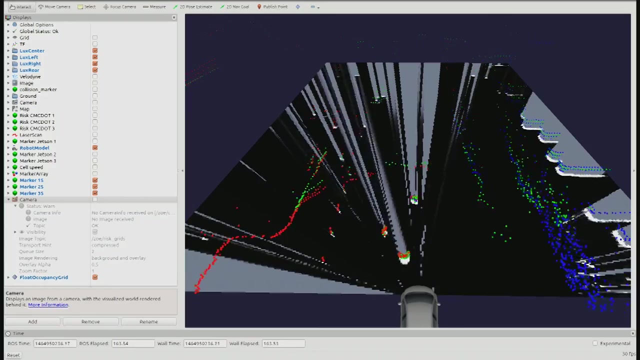 And, on the other hand, to be able to remove ambiguities, as when you have a sequence of images of a scene, you understand what is happening much better And you can remove certain ambiguities and correct certain errors of perception. But we have also manufactured a much more compact perception box. 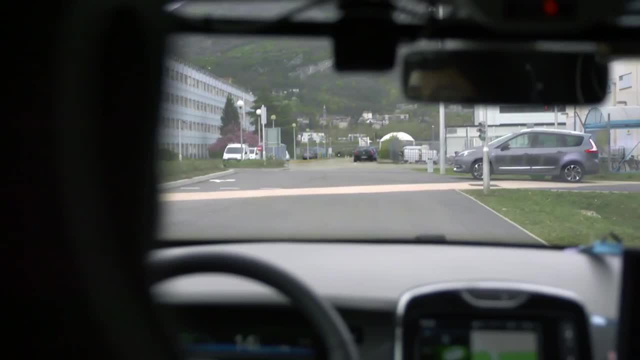 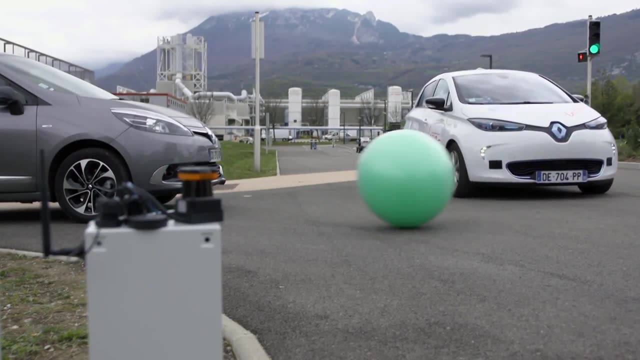 which can be positioned at intersections, Or you can put it in a bus in order to be able to detect pedestrians which cars couldn't see, And so in this box, we sort of replicate what is in the vehicle in a much more simplistic fashion. 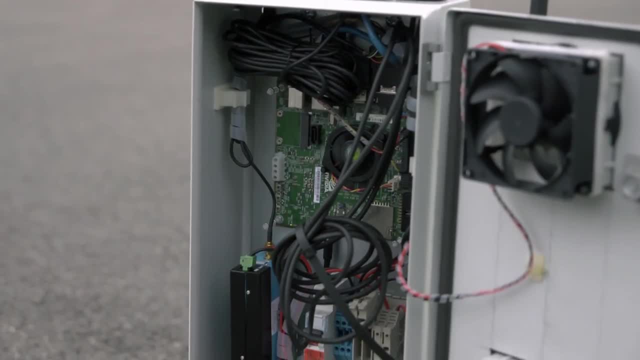 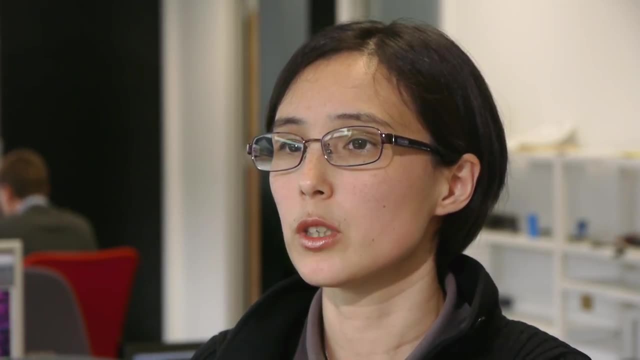 So there is only one leader, for example, in the box, a GPS, an embedded board, of course, in order to process the data, and a geo-networking box. With this box, which can be considered as a Wi-Fi network, we'll send information from the box to the car. 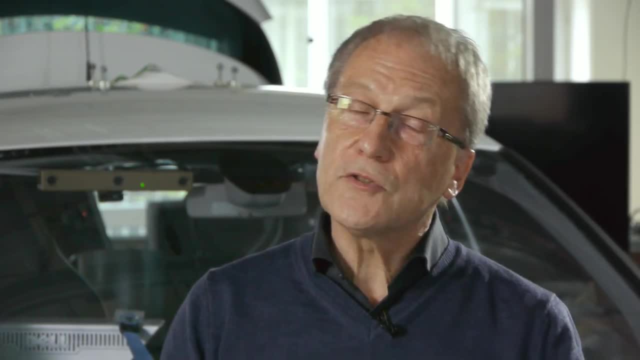 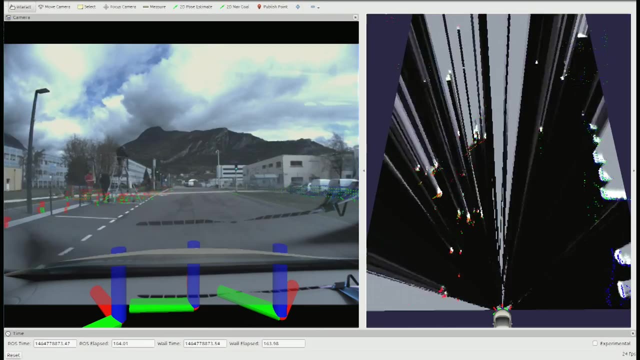 The concept of temporal reasoning and, above all, of prediction is extremely important. If you look at any driver and what they do, they are constantly doing that. They look at the scene in front of them, they understand it and they predict what will happen in the following seconds. 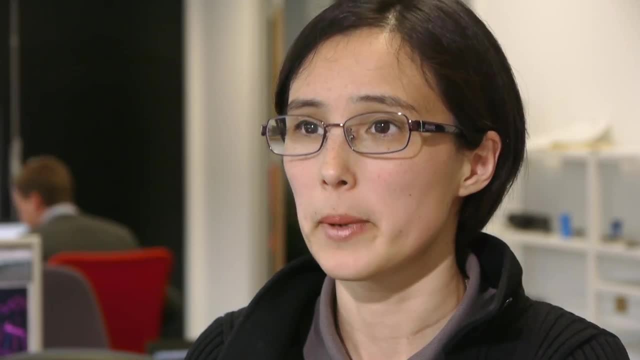 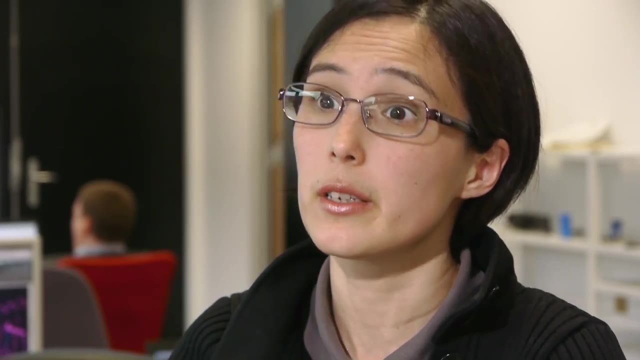 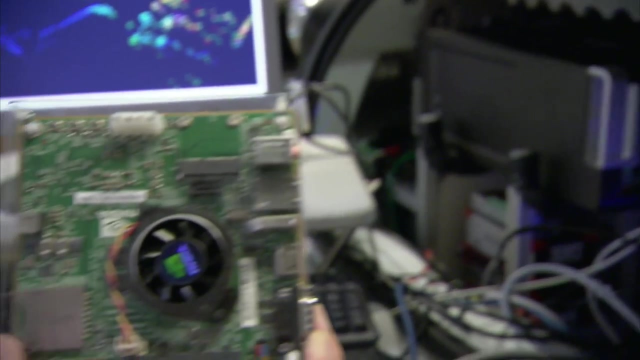 The PERFECT project focuses on all these algorithms of perception in order to allow the vehicle to navigate autonomously in cities and avoid hitting pedestrians, And one of the keys at IRT NanoELEC is to miniaturize the hardware as far as possible.